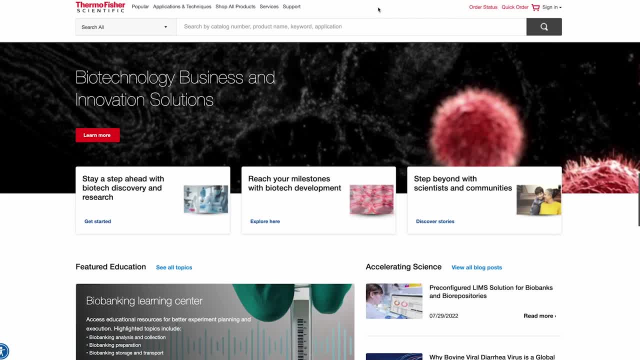 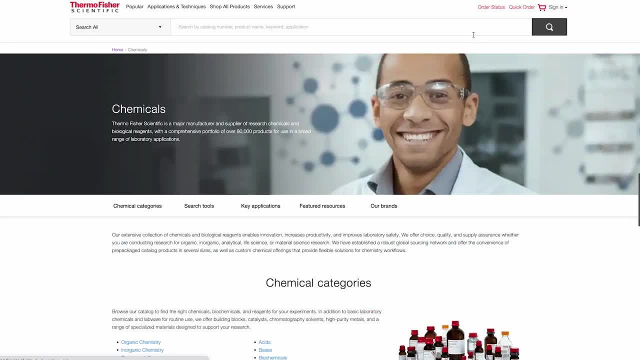 This video is brought to you by Thermo Fisher Scientific. Offering a wide range of reagents and materials, Thermo Fisher supports virtually every laboratory application, from research to drug discovery and development to manufacturing, With over 80,000 laboratory chemicals now on one. 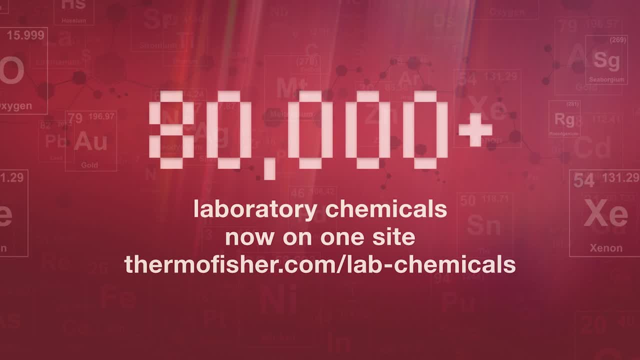 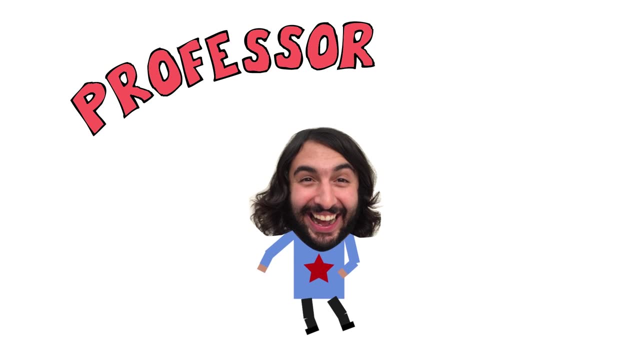 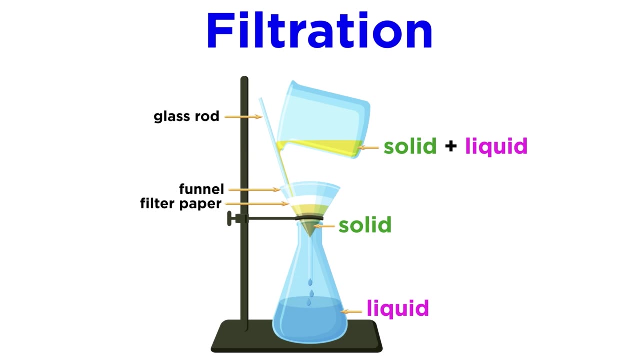 site, Thermo Fisher delivers choice, quality and supply assurance for all your chemical needs. Visit the link below for more information. In the previous tutorial, we learned about filtration, a technique that allows us to separate solid and liquid components of a mixture. But what if the components we wish to separate are 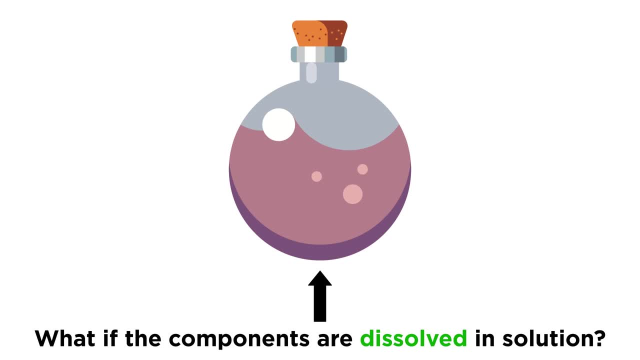 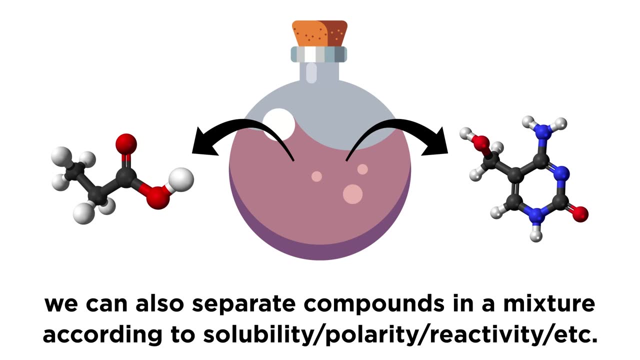 both in solution. There is nothing about particle size that will allow us to do so. Fortunately, there are separation techniques in chemistry that take advantage of factors other than particle size in order to separate components. These focus on properties such as solubility, polarity and reactivity. 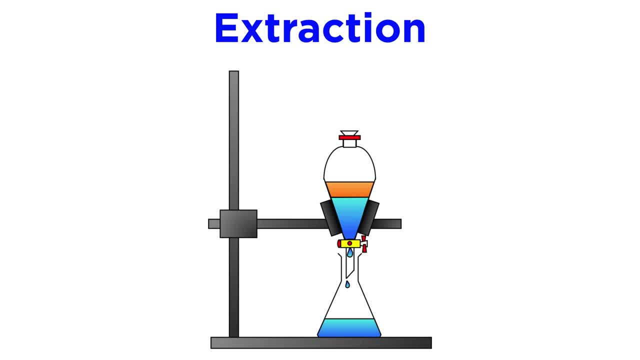 The technique we will go over in this tutorial is called extraction. Extraction is a technique that uses a two-phase system to separate mixtures. The most common form is a liquid-liquid extraction and in this context, the two-phase system will be an organic phase and an aqueous phase. 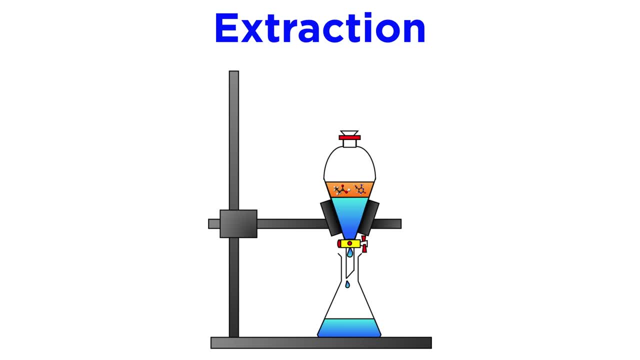 So in performing this technique, we will separate a desired compound from a mixture by moving it from the liquid to the liquid and then separating it from the liquid to the liquid. So in performing this technique, we will separate a desired compound from a mixture by moving it from. 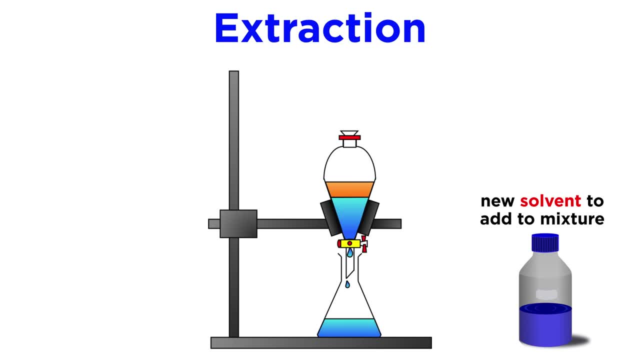 one solvent to another. To perform this technique. we will be taking the solution and adding a new solvent that dissolves and isolates one compound from the mixture. We must use a solvent that is immiscible with the first solvent so that separate layers will form, as this makes it quite easy to 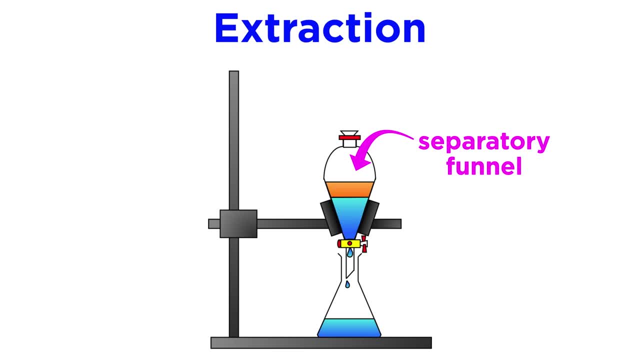 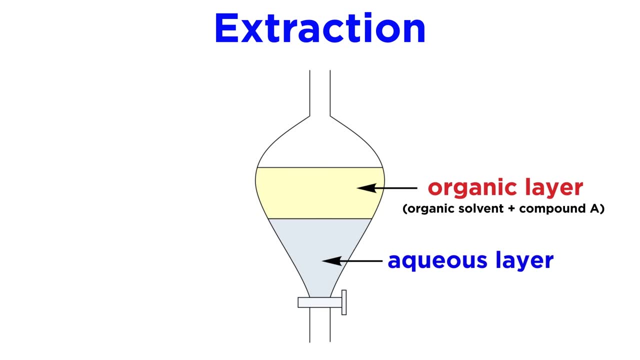 separate them. To do this, we'll need a separatory funnel. This is a tool that is used to separate two immiscible liquids of different densities. Once again, in most cases, the two liquids will be an organic solvent plus whatever compounds are dissolved in it, and then water plus whatever. 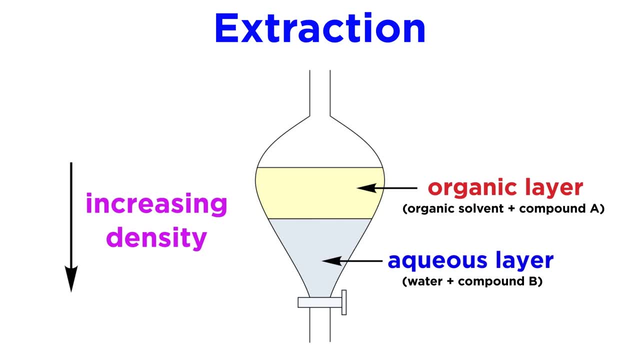 compounds are dissolved in it. It is usually the case that the aqueous layer has a greater density than the organic layer, so it goes to the bottom while the organic solvent stays on top, as gravity will pull the denser layer down with greater force. 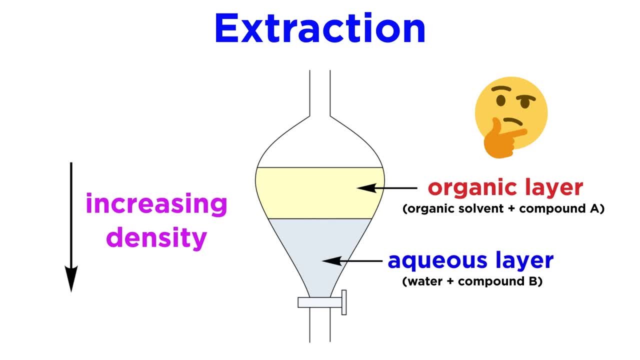 However, some organic solvents are more dense than water and will thus occupy the bottom layer. so it is important to consult a table of densities to be sure as to which layer is which When in doubt. if you want to identify which layer is which, add a bit of water. 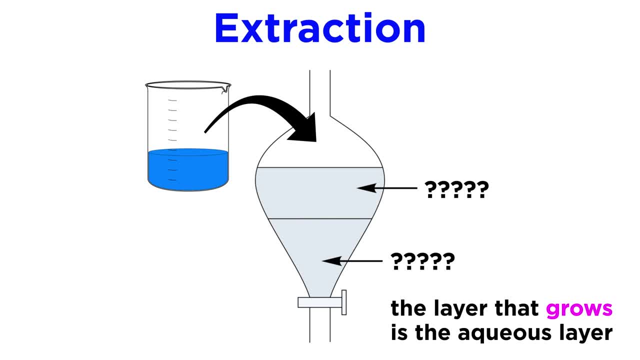 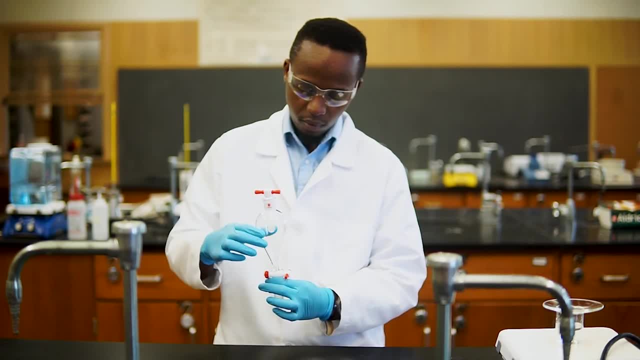 Whichever layer grows, that's the aqueous layer. Now let's get more familiar with the intricacies of the separatory funnel. As we can see here, the funnel has a stopper at the top and a stopcock at the bottom. This middle region is where our separation will take place. To get this ready, 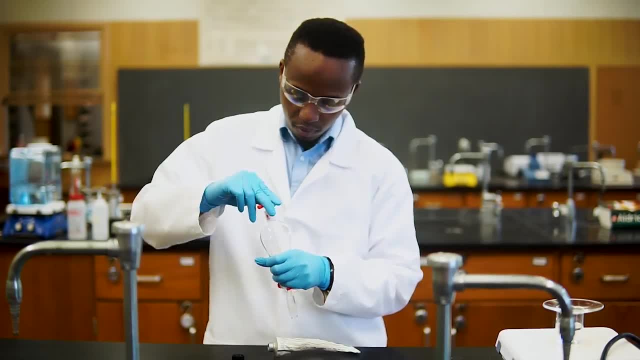 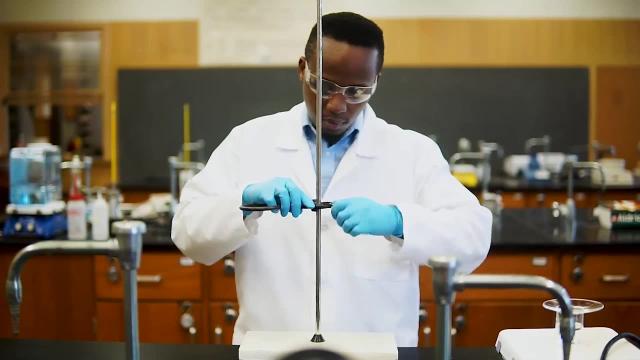 you might have to add a little bit of grease to the stopper and or stopcock, since they tend to get stuck To set up for the extraction. we'll start with the top layer and then we'll add the ring stand attached to a support like this. We'll then place our separatory funnel in the ring and 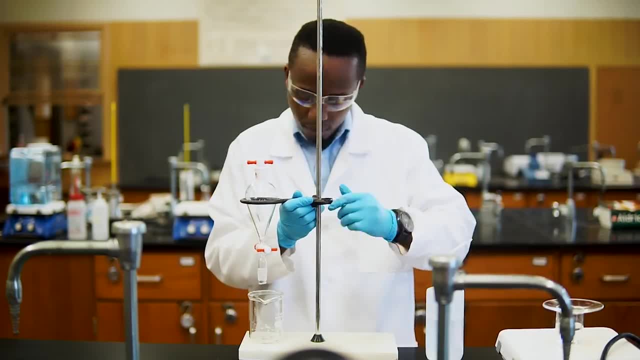 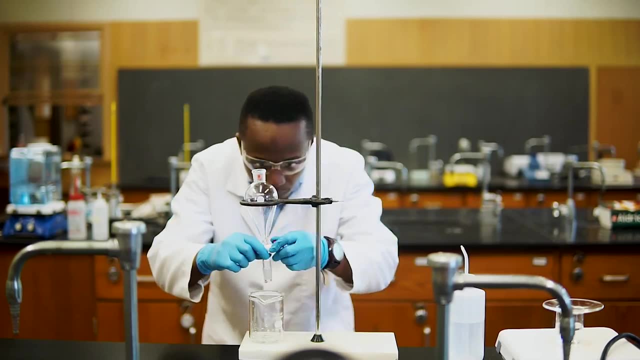 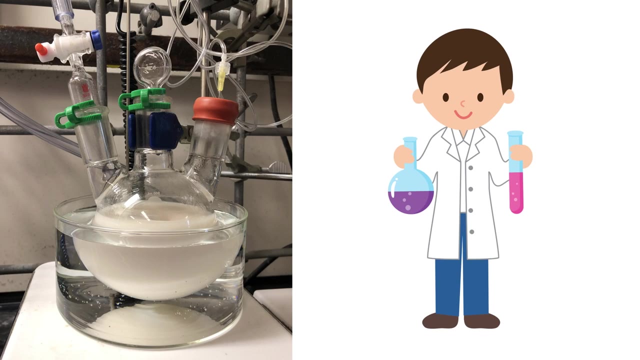 make sure everything is secure. To verify that the stopcock works, add some water. Make sure there are no leaks when the valve is closed. Open the valve to see how the water flows. Once satisfied, remove the water. We are now ready to get started. So let's say this is a reaction mixture that we 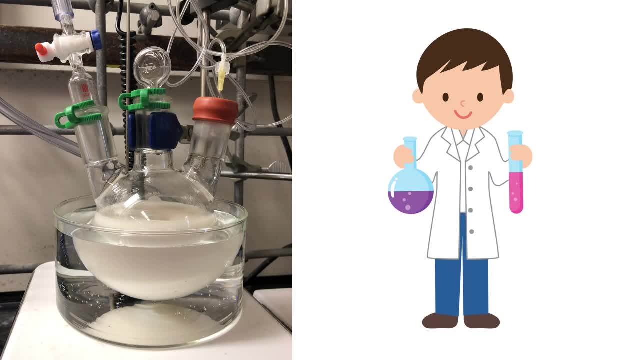 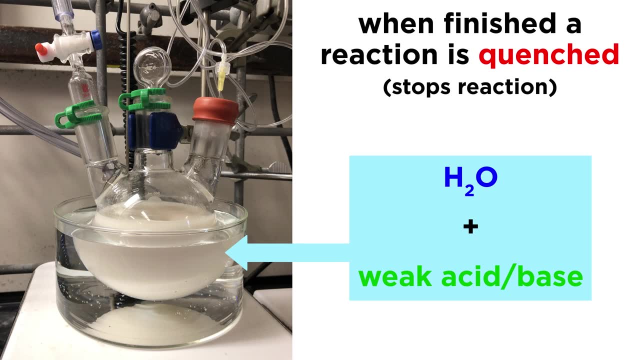 just got from performing a chemical reaction in some organic solvent. Most of the time you'll need to quench a reaction once it's finished by adding water. This means to stop a reaction mixture from reacting further, often with dilute weak acid or base to neutralize any 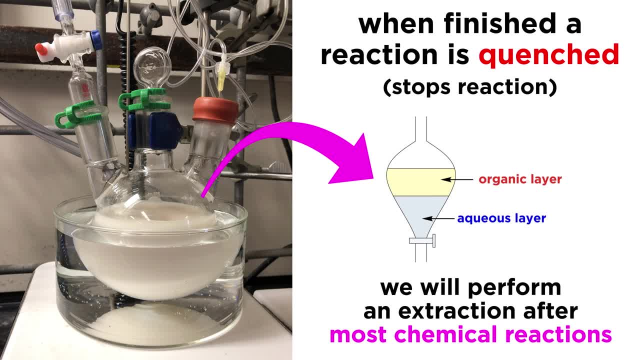 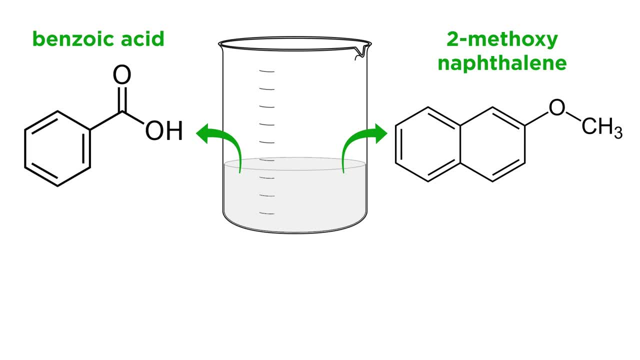 ionic species. This means that after any chemical reaction, you will need to perform an extraction to separate your organic compounds from whatever is in the aqueous layer. In this particular case, rather than a reaction mixture, we simply have a mixture containing benzoic acid and 2-methoxynaphthalene. 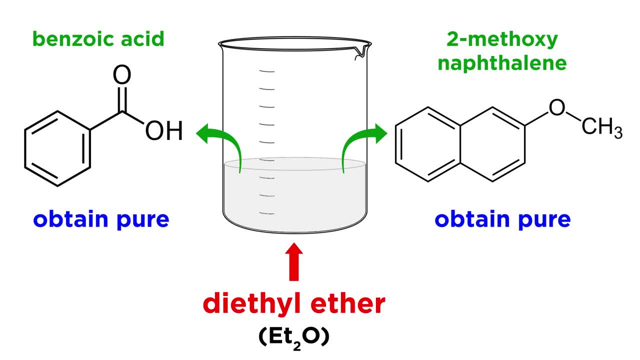 dissolved in the solution. This will help the reaction mixture to be more stable and more soluble in diethyl ether, and our goal is to obtain each of these two compounds in a pure form. These are both soluble in diethyl ether but insoluble in water. However, if we add aqueous, 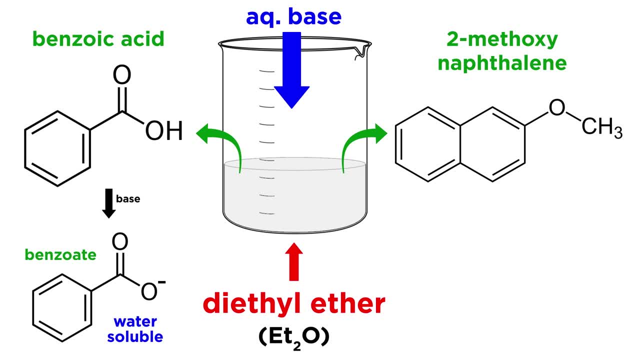 base to this mixture, benzoic acid will deprotonate, becoming the benzoate anion, which has a formal negative charge, and will thus become water-soluble and move into the aqueous phase. Since 2-methoxynaphthalene will not react, that will remain in the organic phase. 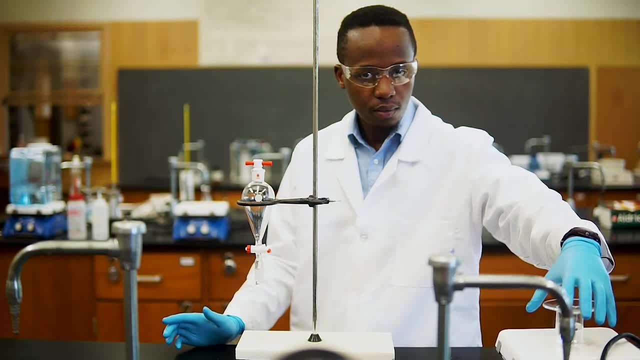 and the two compounds will be soluble in the aqueous phase. Since 2-methoxynaphthalene will not react, that will remain in the organic phase and the two compounds will be soluble in the aqueous phase. With our strategy understood, we can begin performing the technique, Making sure that 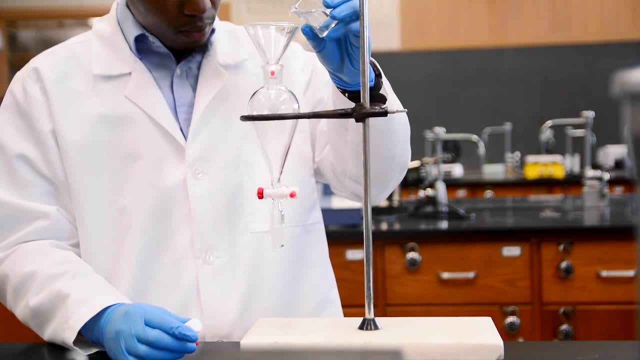 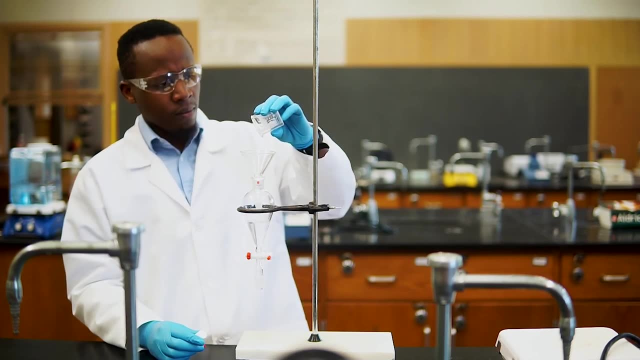 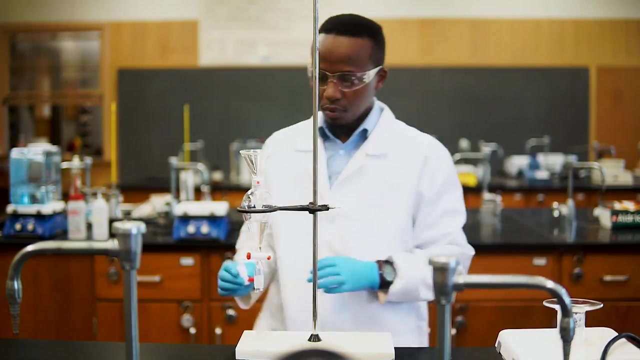 the stopcock is closed. let's transfer our mixture to the separatory funnel using a conical glass funnel. This is our organic layer. To make sure we have transferred everything, rinse the beaker that held the mixture with ether and transfer that as well. Had this been, 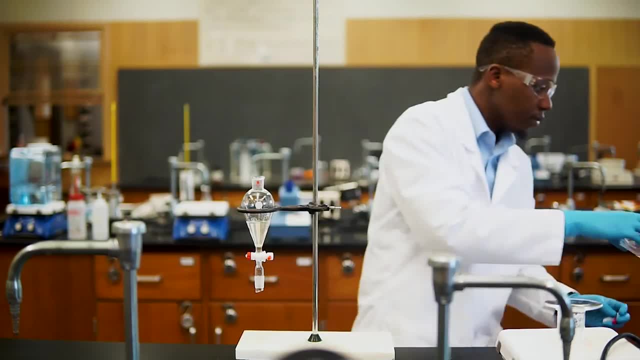 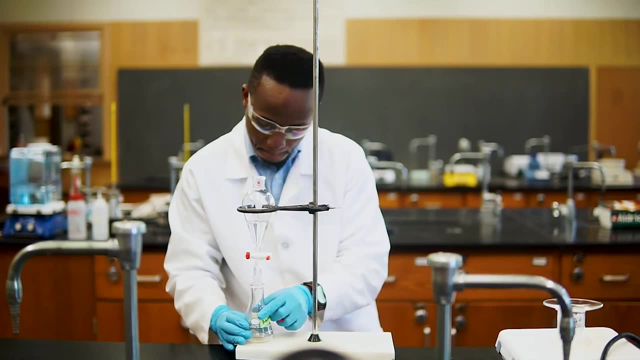 the product of a chemical reaction. it would already have been quenched and thus have formed. but since we are just doing an isolated extraction, let's go ahead and perform the necessary acid-base reaction right in the separatory funnel To separate benzoic acid. 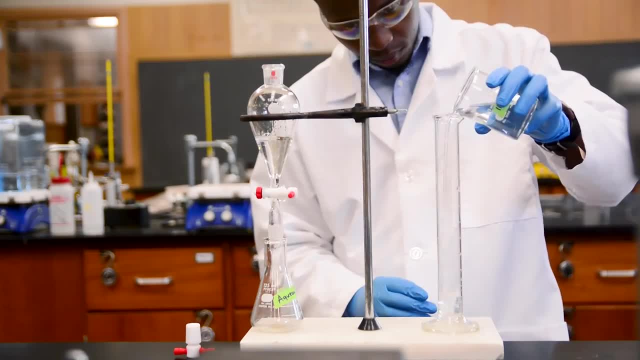 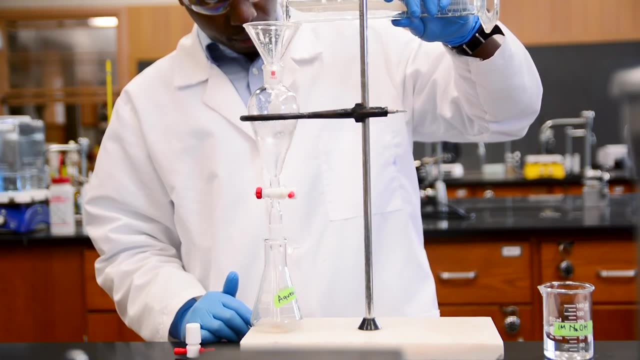 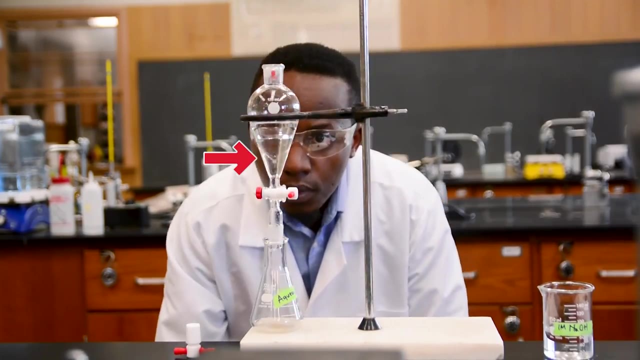 from the mixture. we will add 30 milliliters of 1 molar sodium hydroxide to the separatory funnel. This will pass through the organic layer, react with benzoic acid on the way to form sodium benzoate and drag that down to the newly forming aqueous layer on the bottom. 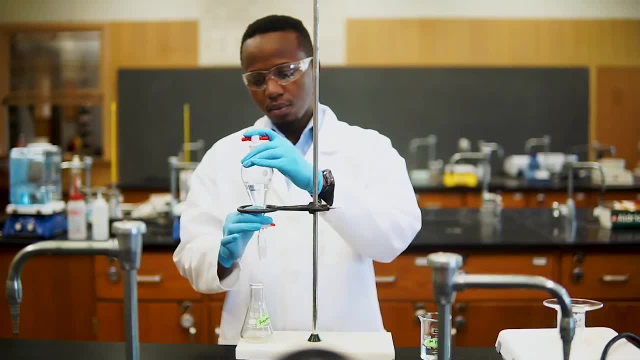 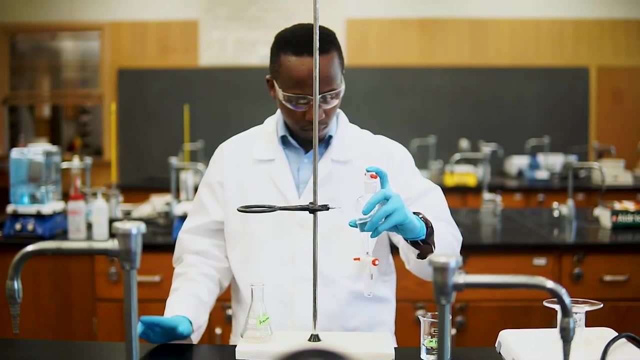 To make sure the reaction goes to completion, we need to mix the contents of the funnel. We will do this by inverting it and lightly swirling a few times, holding the stopper down with one finger as we do so to ensure that nothing spills out. Mix for about 10 seconds each time. 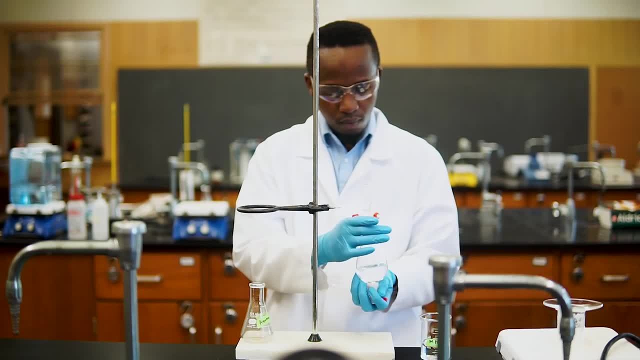 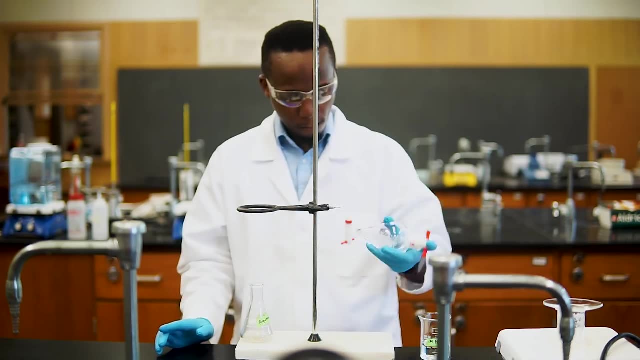 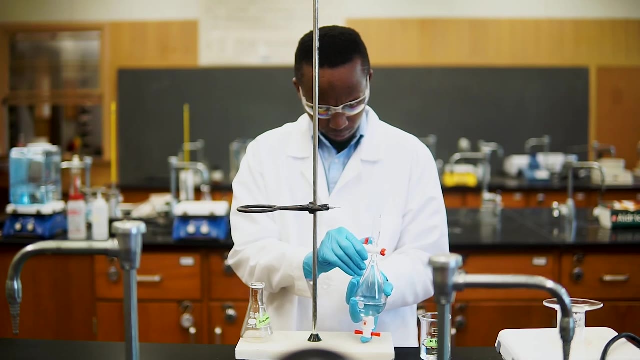 After each round of mixing, hold the funnel upside down and open the stopcock like this to vent any gases that accumulate from the reaction, Close it and then continue mixing. When gas is vented, you will hear a brief hissing sound. When the sound no longer occurs, 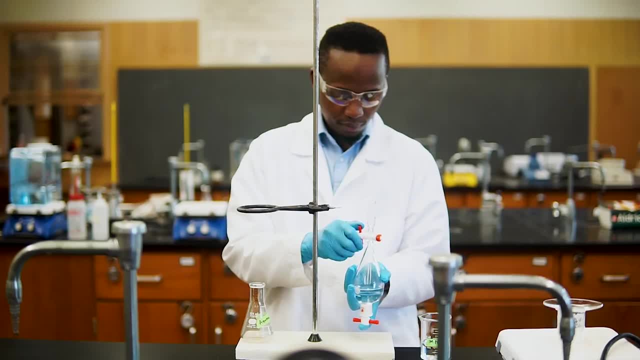 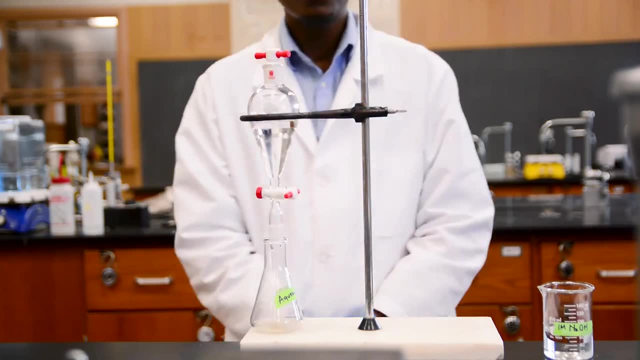 no more gas is being produced and we can be confident that mixing is complete. After mixing, it is time to separate. Return your separatory funnel to the ring support and allow the contents to settle. You should see the two layers separate clearly. 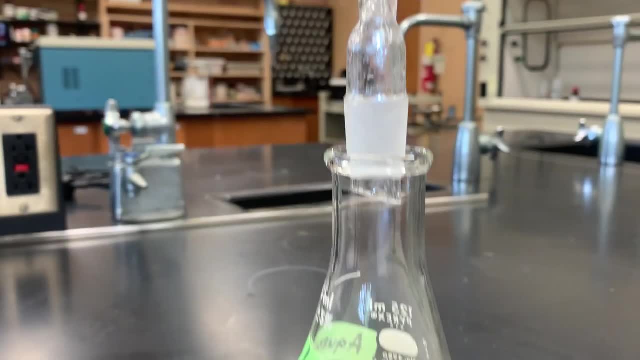 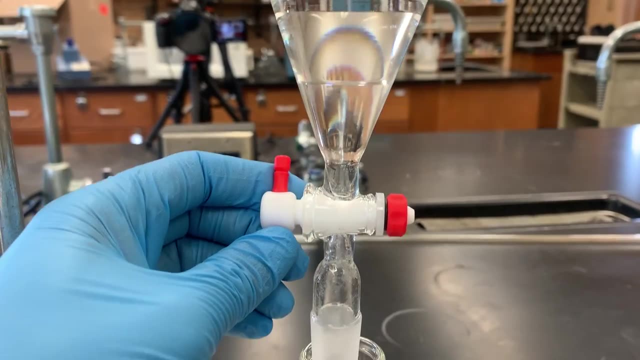 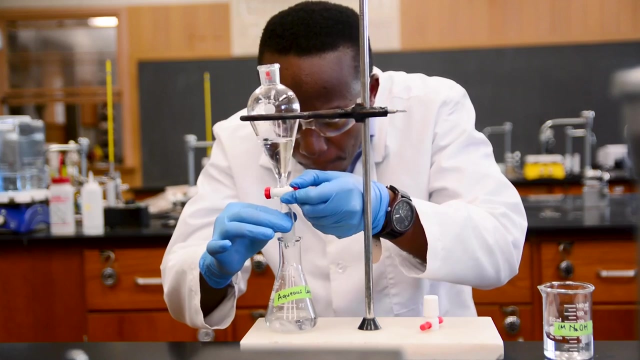 You can now open the stopcock to let the bottom layer drop into a clean flask. This is where you have to be careful. Watch the aqueous layer drip slowly so that you can stop it right before any of the top layer goes through. When the line separating the layers reaches the stopcock, close it. You have now separated the. 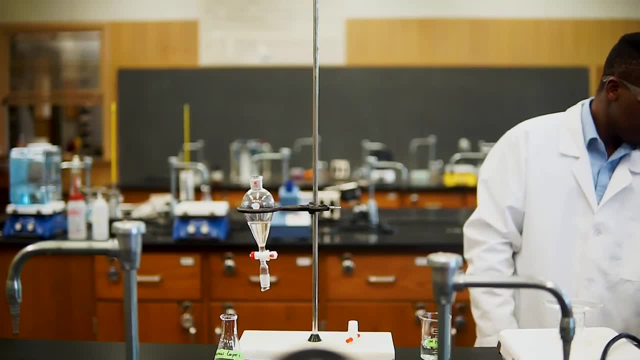 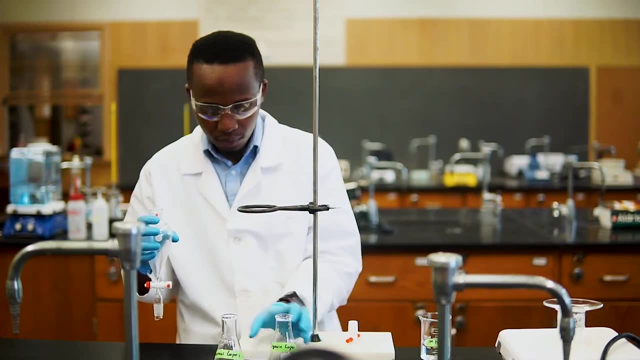 two layers. The top layer can be removed by pouring it through the top of the funnel into a separate flask. Be sure to pour it out the top and not through the stopcock, as pouring out the bottom would contaminate it. With most extractions we will need to do more than one separation, so as 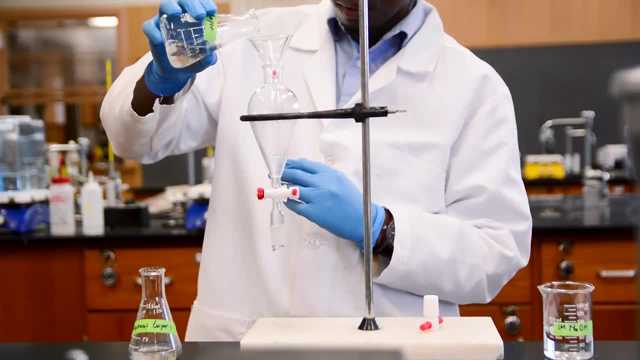 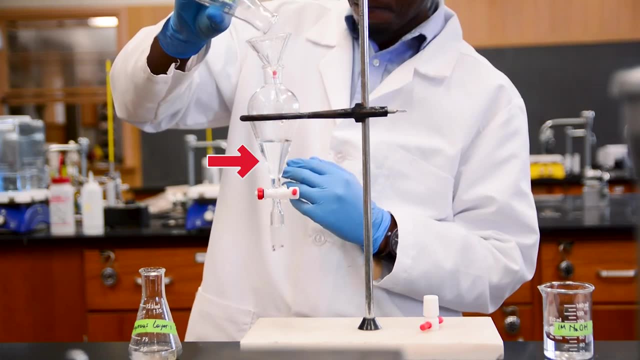 to maximize your yield. If the top layer goes through the stopcock, the top layer will not be able to separate, as not all of the benzoic acid made it out of the organic layer. So let's put this first aqueous extract to the side. return the organic layer to the separatory funnel. 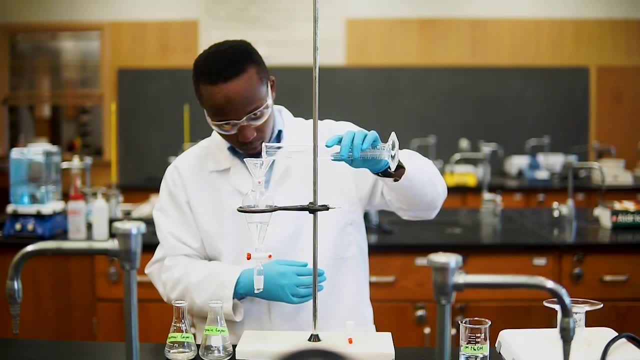 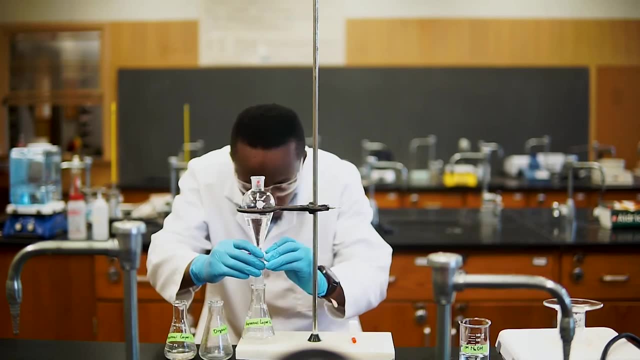 and make sure everything is secured. We can then add more aqueous base to the organic layer and mix just as we did before, Allow the layers to separate and we can now collect the bottom layer again, adding it to the original extract. 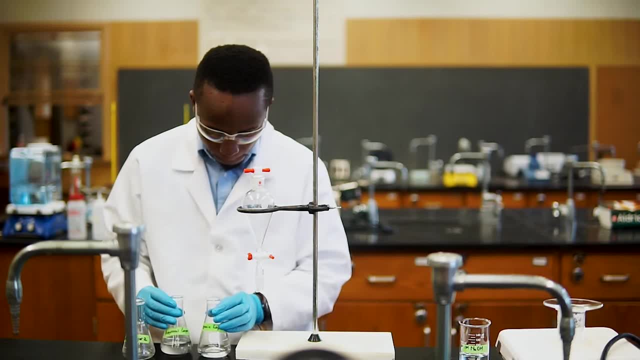 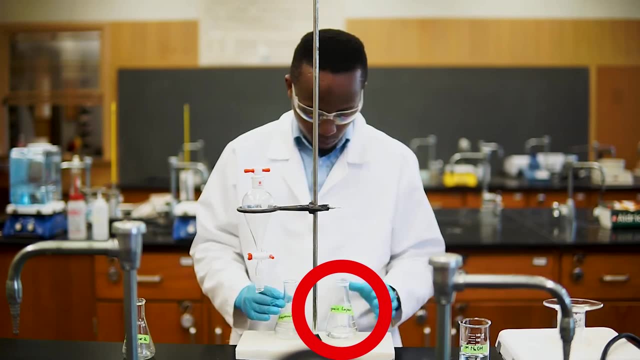 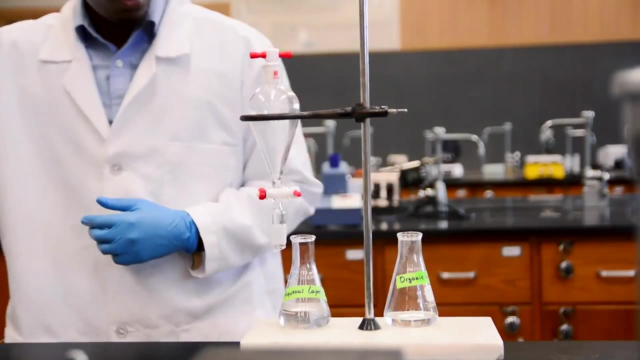 So now the extraction itself is complete. We have some aqueous sodium benzoate, and then we have two methoxynaphthalene still in the organic solvent. Let's isolate this first. The organic layer will likely contain residual water from the multiple washes that we performed. 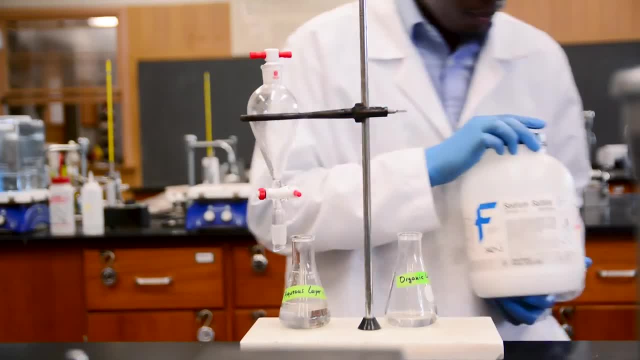 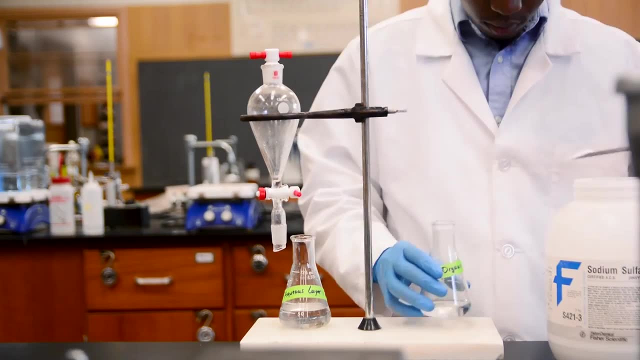 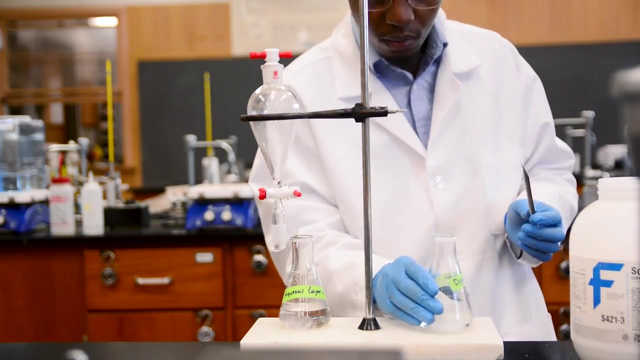 How do we get it out? We use a drying agent. A drying agent is a compound like sodium sulfate that removes water when added to a solution. The water should bind to the solution. and the water should bind to the solution- the drying agent- and thus join the solid phase. Keep adding the drying agent until you see a clear. 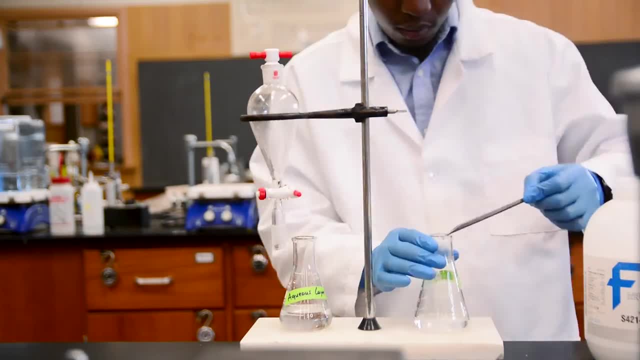 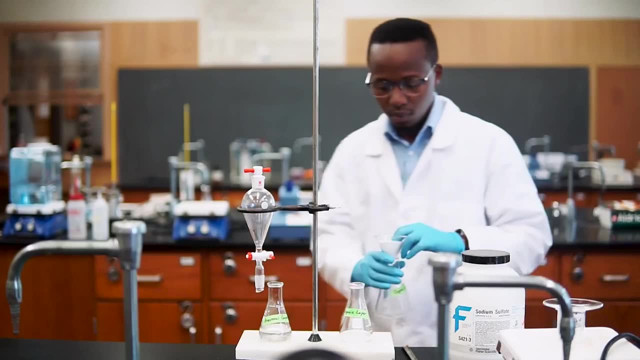 solution with all of the solid clumped at the bottom. You will know it's dry when lightly shaking the flask does not cause any solid to move around the solution. To separate the drying agent from the liquid we'll need to do a gravity filtration. Since we discussed this at great 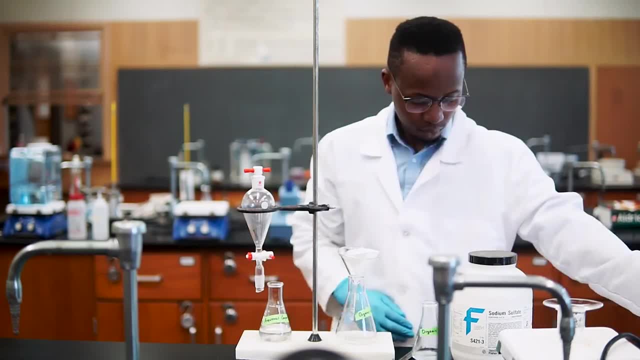 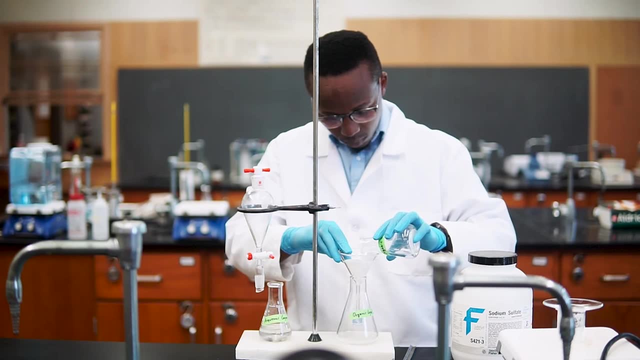 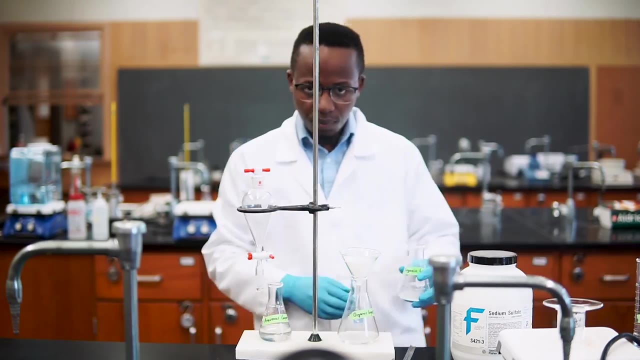 length in the previous tutorial. we won't go over the details here, but set up your filtration and pour your dried organic layer in The drying agent will remain on the filter paper and the target molecule will move through with the solvent. Make sure to rinse the flask with more solvent so that everything is transferred. 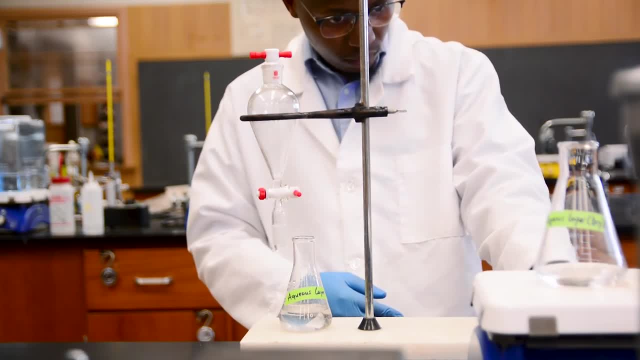 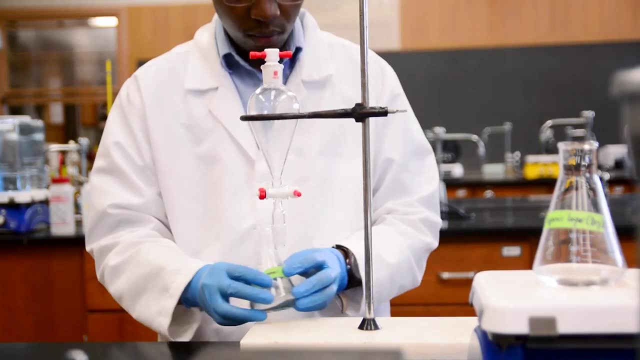 Then just evaporate the solvent on a hot plate, as ether is rather volatile, and we will be left with the residue of pure two, methoxynaphthalene. The aqueous layer will be a bit trickier, as we wanted to isolate benzoic acid.